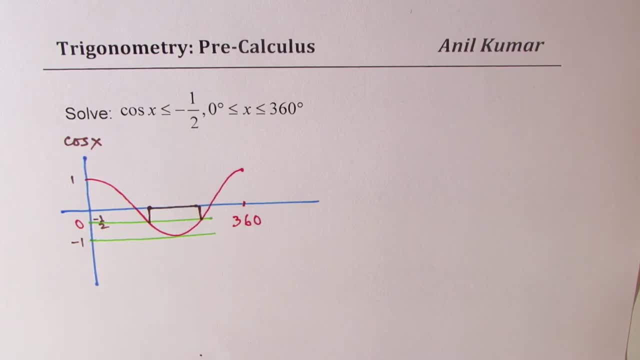 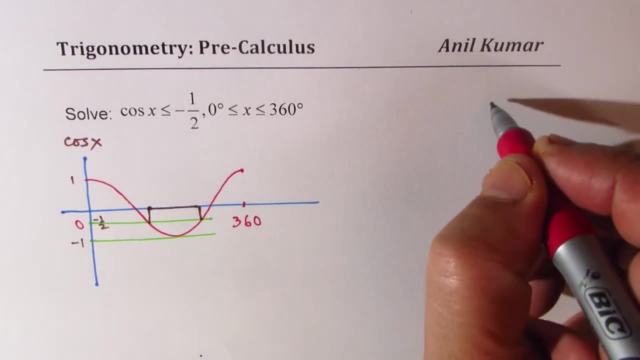 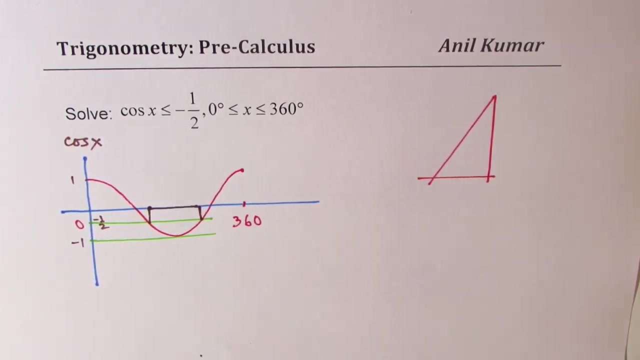 So what remains is to figure out when is cos x half right? For that we could actually sketch the special triangle. So let's say this is the special triangle. Some of you can also take help of calculator, But in these tests calculators are not allowed, right? So let's be very clear. 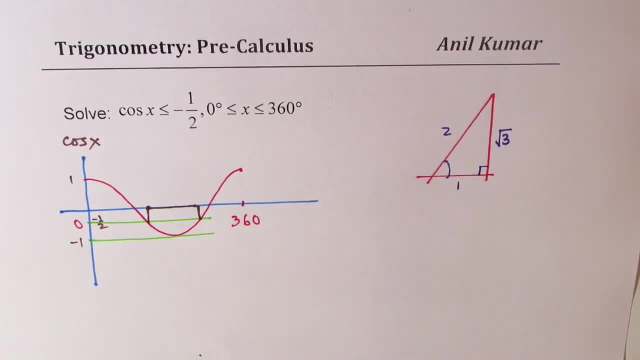 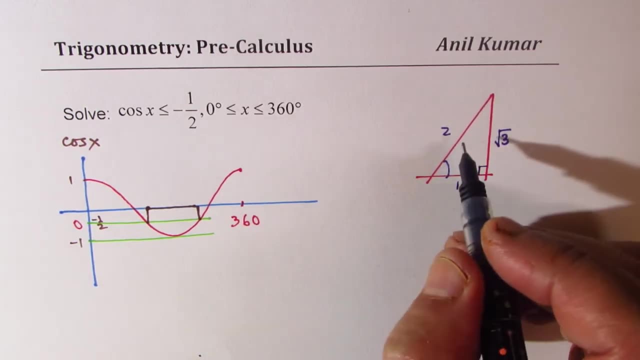 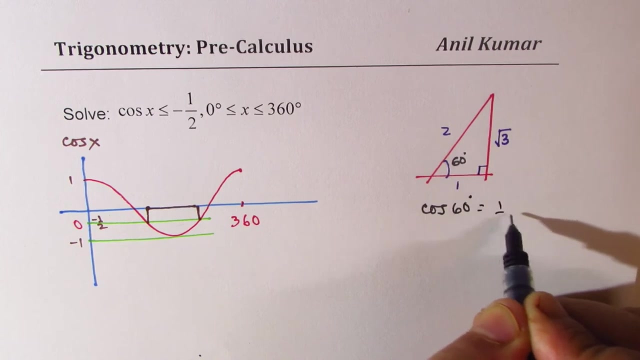 about it. Now for this triangle, which is 30, 60, 90, we know that cos x is less than equal to minus half right. So this is 60 degrees, that is 90. In that case, we know cos of 60 degrees is. 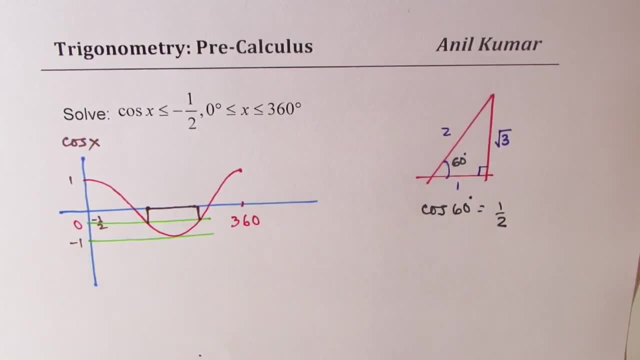 half Now. since it is negative, it really means that we are in quadrant 2 and 3, right, So that is the rule. All are positive here sine tan and cosine, So cos is negative in quadrant 2 and 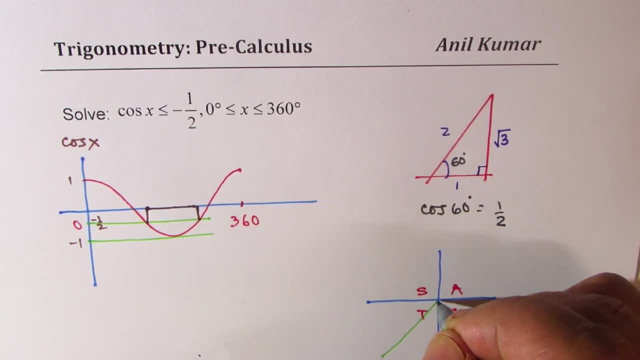 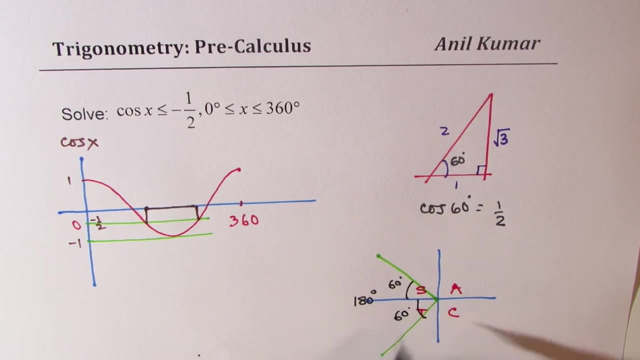 3. So we are looking for these two values right? So at these two values, cos is negative. So if this is 180 degrees, here the angle is 60 degrees, acute angle, correct. So cosine is: 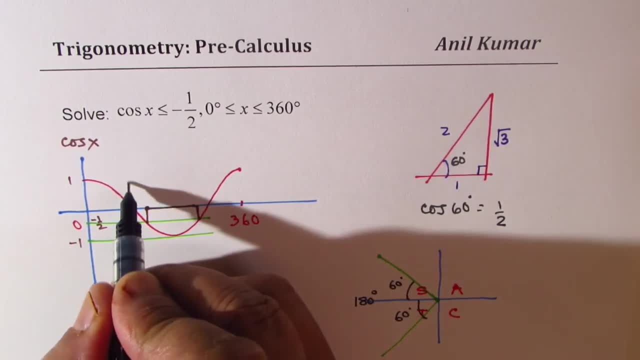 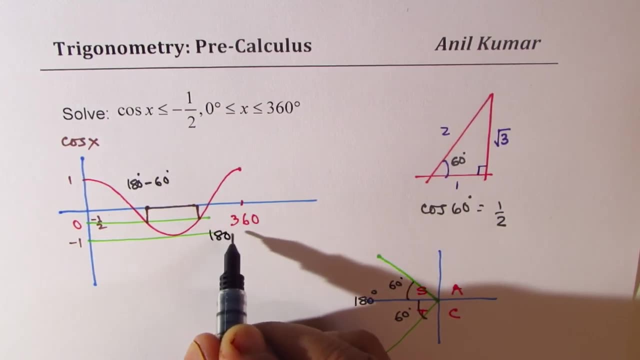 negative. So what we find? that this is 180 degrees minus 60 degrees And the other one is 180 degrees plus 60 degrees, correct? So the x value is basically between 180 degrees minus 60 degrees and 180 degrees plus 60 degrees, correct? So we have our solution. 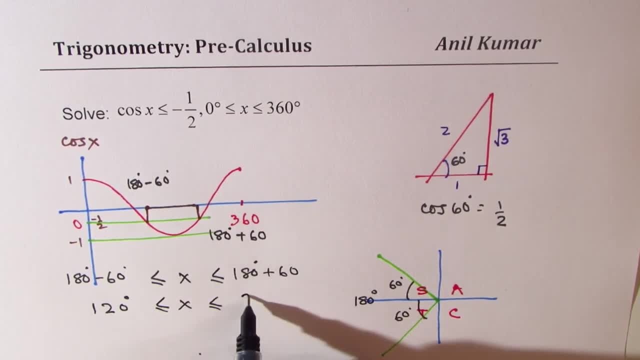 right there: 120 degrees to 240 degrees. So that becomes the solution of the given question. So I hope it makes sense. Correct. So cos x is less than minus half, as you can see in the interval when x is between: 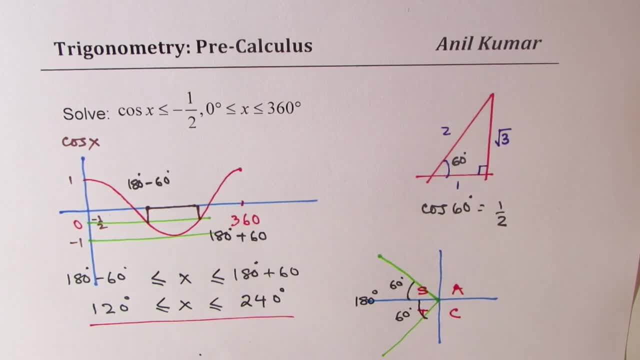 120 degrees and 240 degrees, as shown in this particular solution. Feel free to write your comments and share your views, and I hope that helps. Thanks for watching and all the best.